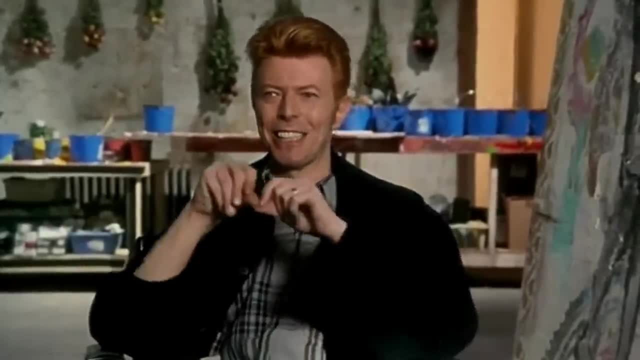 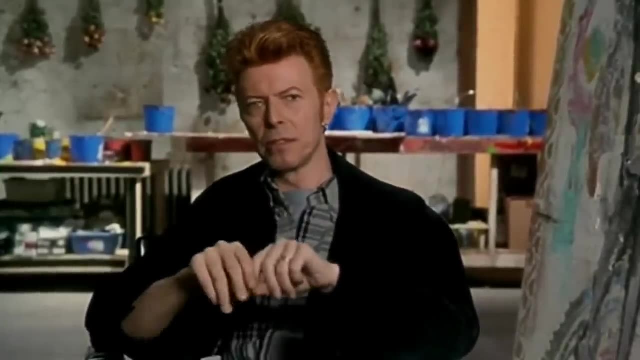 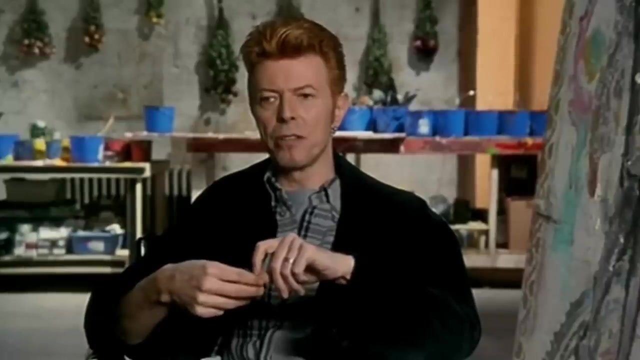 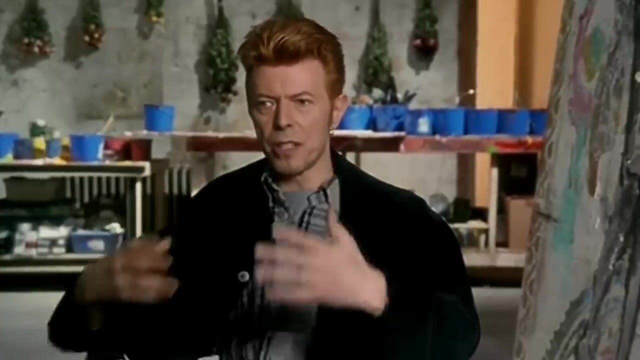 Yes, never play to the gallery, I think, But you never learn that until much later on, I think. But never work for other people in what you do. Always remember that the reason that you initially started working was that there was something inside yourself that you felt that if you could manifest it in some way, you would understand more about yourself and how you coexist with the rest of society. 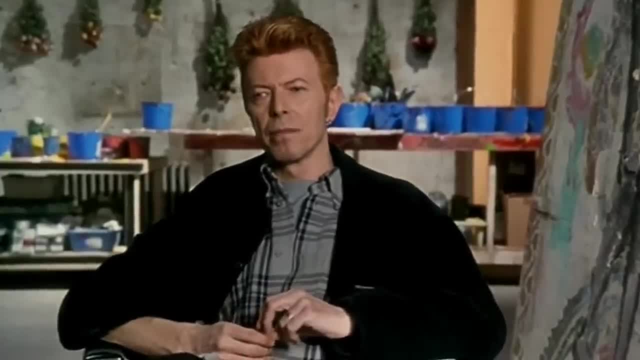 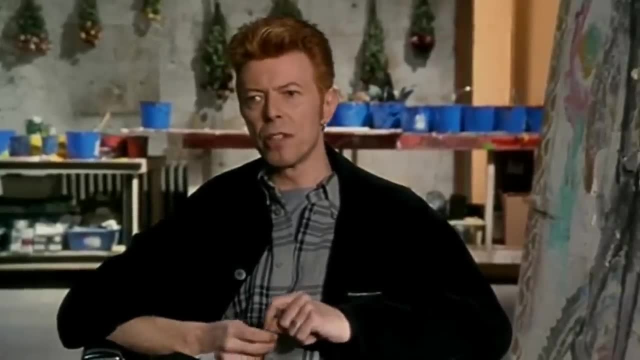 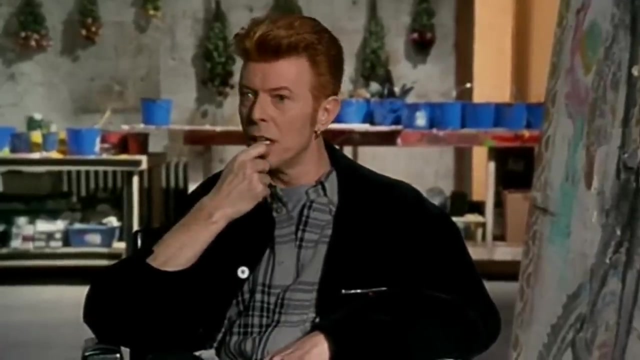 And I think it's terribly dangerous for an artist to fulfill other people's expectations. I think they generally produce their worst work when they do that. And the other thing I would say is that if you feel safe in the area that you're working in, you're not working in the right area. Always go a little further into the water than you feel you're capable of being in. 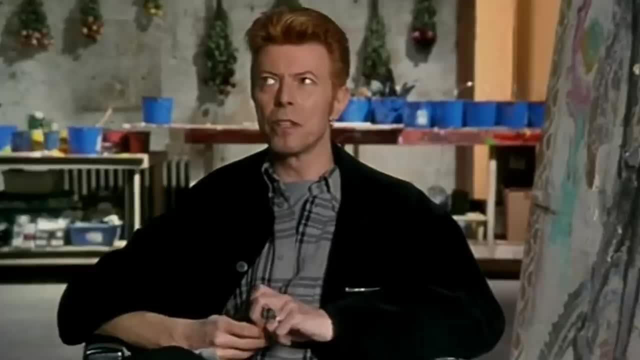 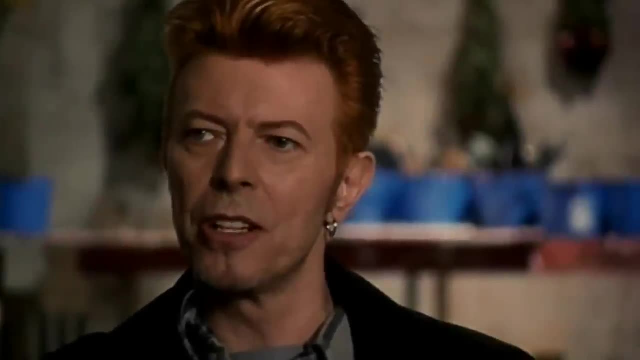 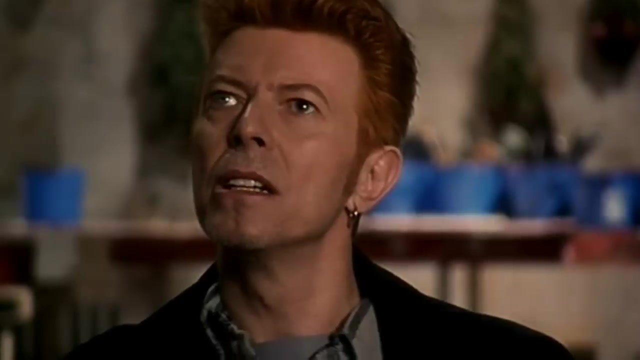 Go a little bit out of your depth And when you don't feel that your feet are quite touching the bottom, you're just about in the right place to do it. Do something exciting. Very much a child and product of the early 60s, it seemed to me to be terribly exciting, and maybe kind of glamorous, to be a commercial artist. 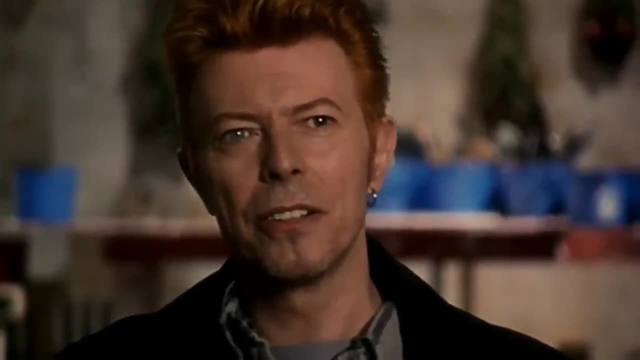 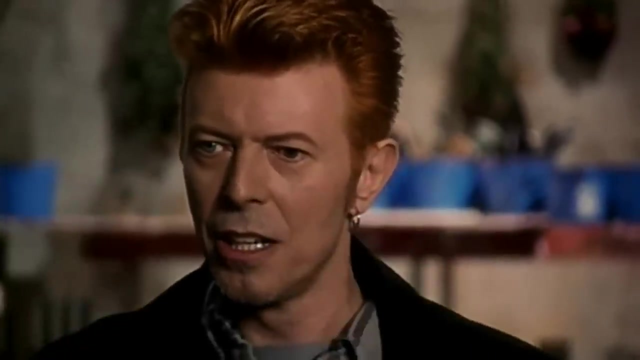 That's what I kind of thought I wanted to do when I was 12.. I thought it must be because I was impressed with things like the father in Dennis the Menace who had those check jackets and the big glasses on, and the crew cut. 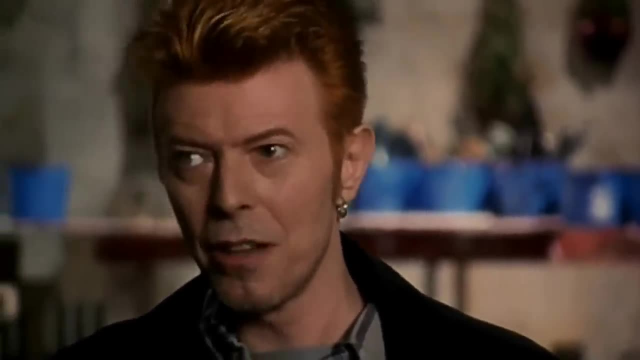 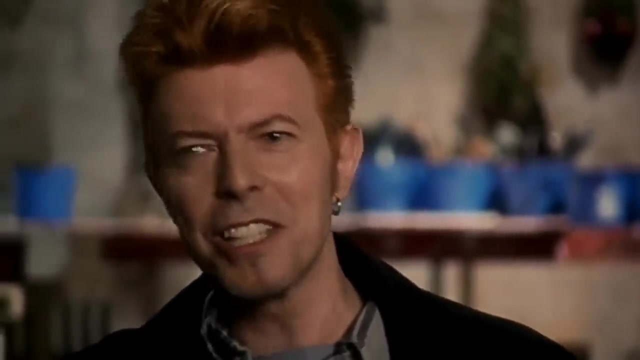 That was a very hip look then, you know, to anybody In Britain. I don't think it was in America, but at the time I thought that's Madison Avenue. you know, that's advertising. that's the place to be. 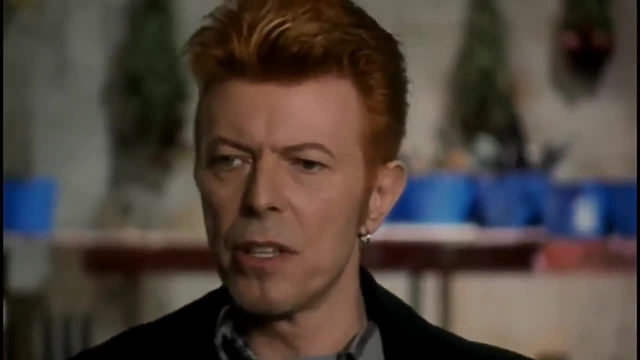 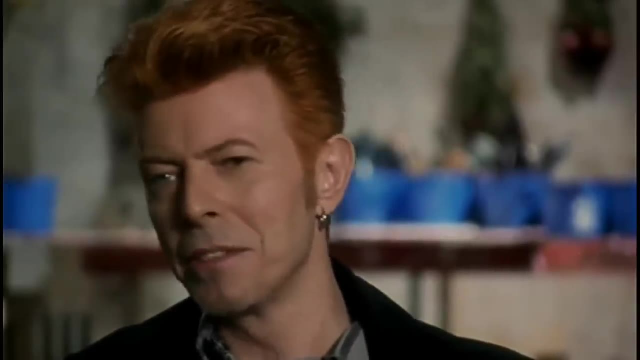 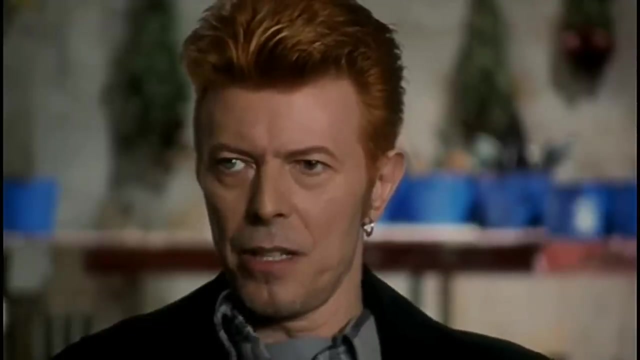 I think the difference that most artists have, the ones that I come across. they think they tend to think we tend to think our opinions are a lot more important than other people's. in some way. Often we feel as though we have the key to something. I don't think that we do at all, I just think we dwell on it more. 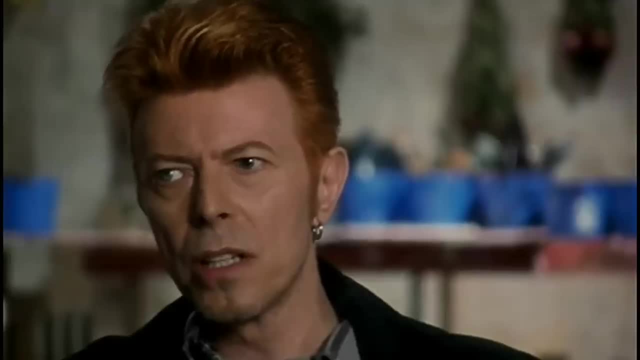 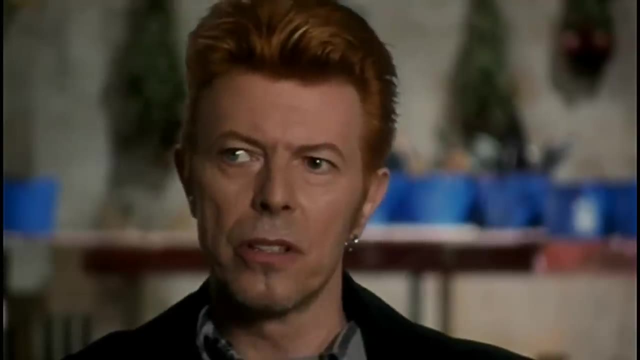 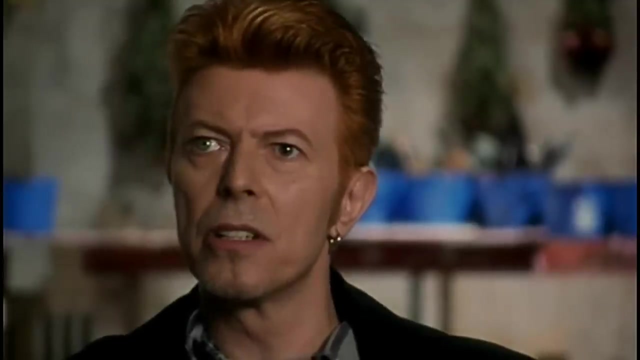 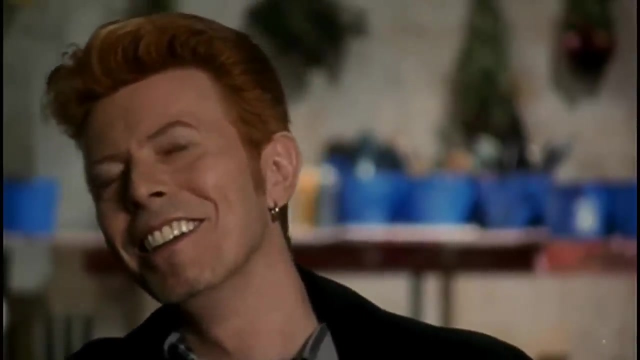 We tend to look at the world as some usable substance- more than a non-artist would, I think. for many people, just getting through life is enough. that's a big enough task, let alone having to look at the world and the universe and say, now, if I had my way, you know. 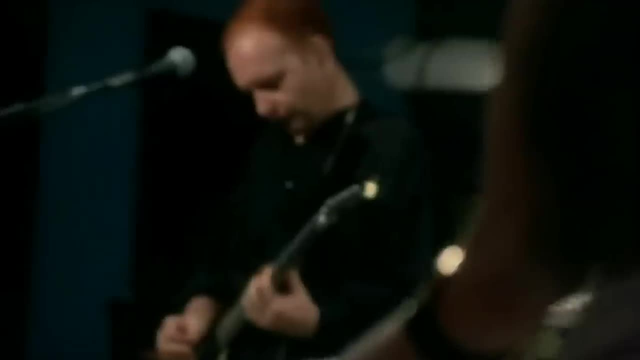 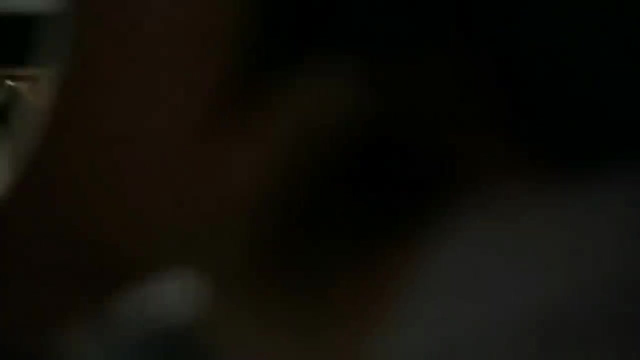 The way that I work, I will either be extraordinarily accepted or otherwise. I reach a point where I've got seven people listening to what I do. I mean, there's never in between, at least, And it's been like that all my life, you know. 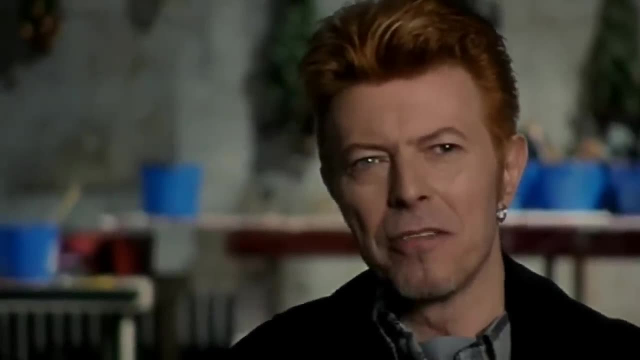 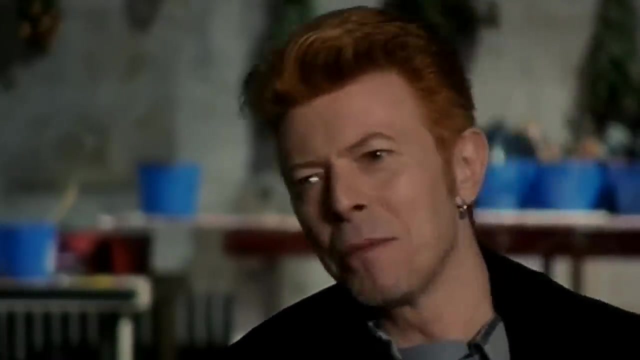 People have either really accepted what I do or they absolutely sort of push it away from them And I guess I've gotten used to that and that's kind of. I guess that's what I am. you know, Sometimes I'm useful currency and other times I'm not. 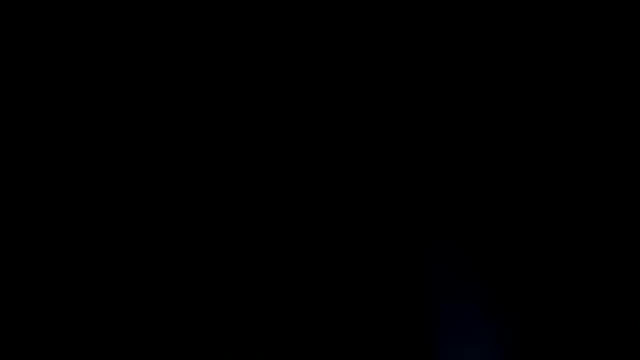 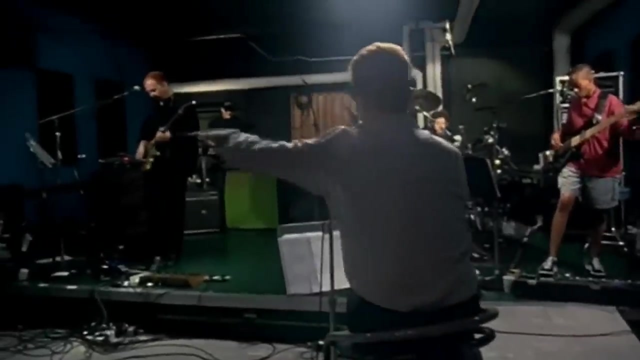 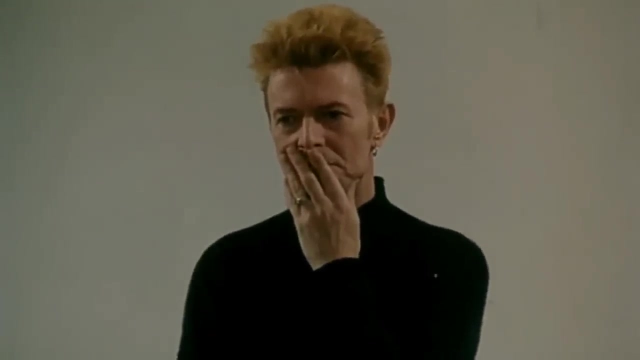 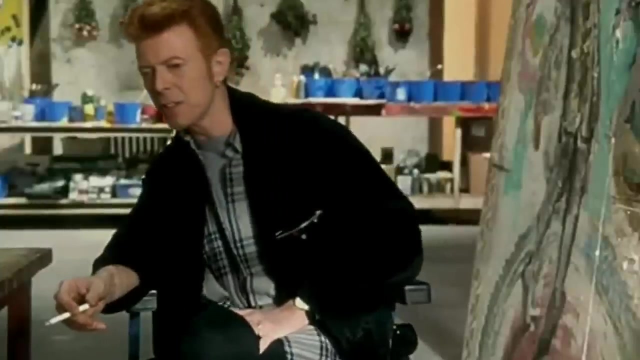 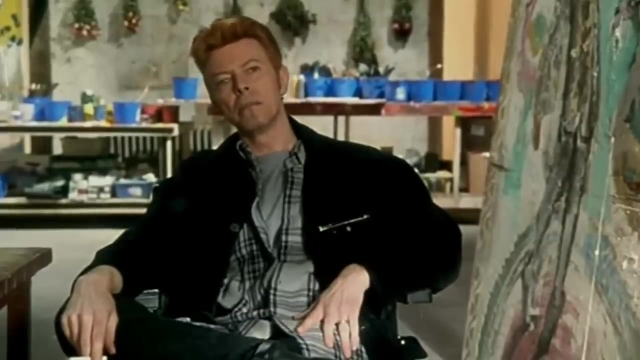 I guess it's all about communication in some ways. How do you communicate those deeper, most feelings that are probably fairly hard to articulate? Well, I think I suppose since I stopped doing drugs and drinking, I think probably I really prize getting up early in the morning, which is something that happens. 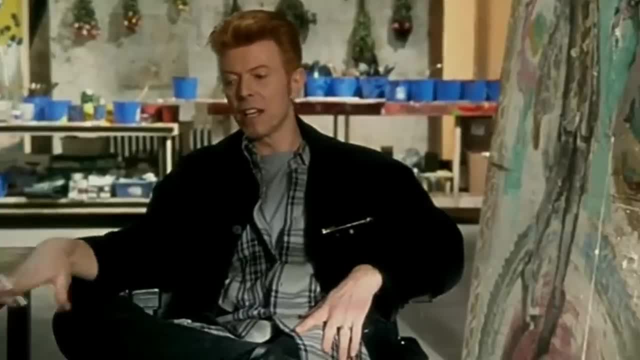 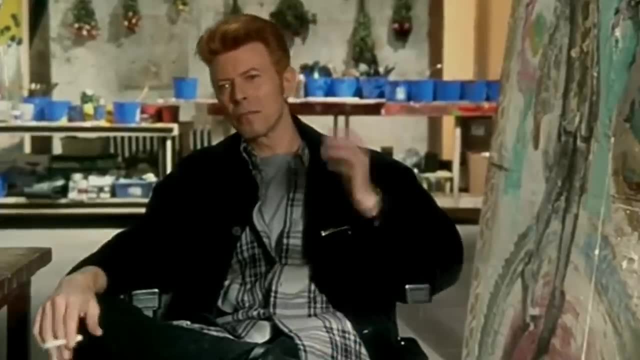 I now find for years now, I've gotten up regularly at six in the morning. It doesn't matter what time I go to bed, I still get up, which is not a great thing actually when I'm rehearsing, because you rehearse pretty late, but I still get up at six. 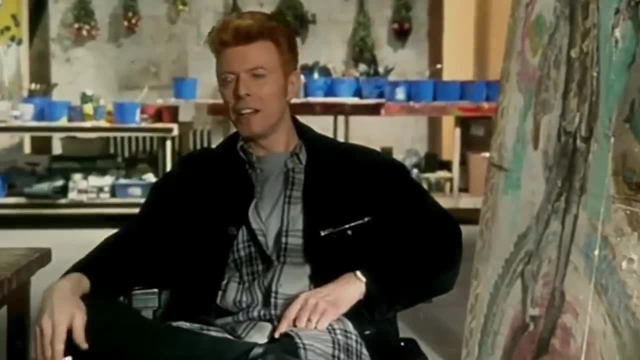 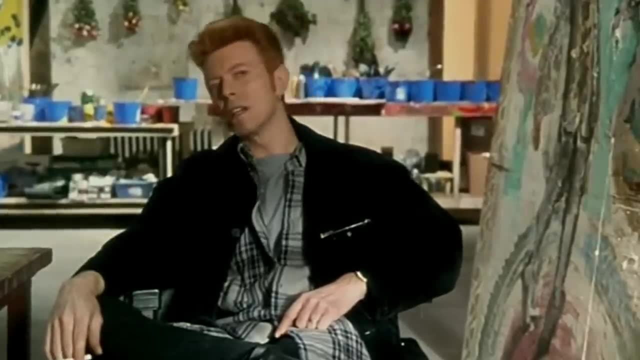 I enjoy the fact of seeing the light come up with me and then utilising the daylight and what it brings and the kind of message that it brings. It's a different message from when you're living in twilight hours and things get very. 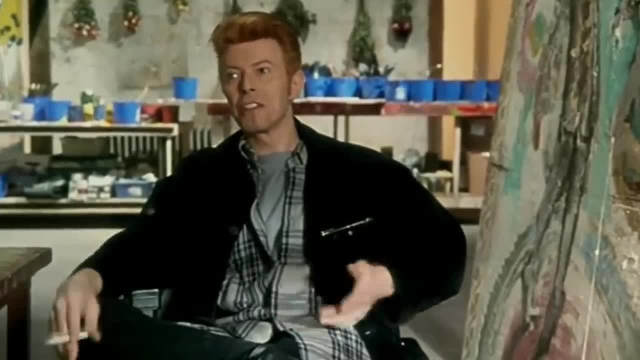 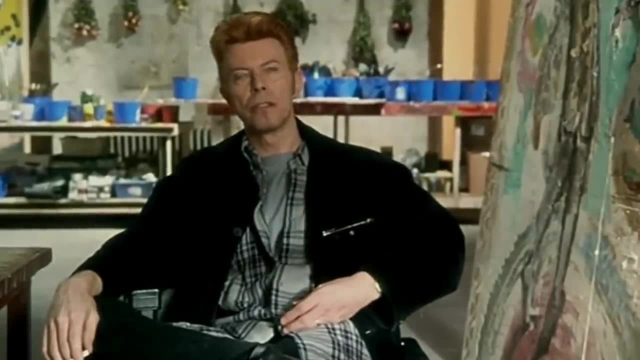 symbolic, representationally, If you live through the twilight hours and the early hours of the morning, there's some kind of there's a shadow to your life all the time. Psychologically you're in the dark as well as physically in the dark. 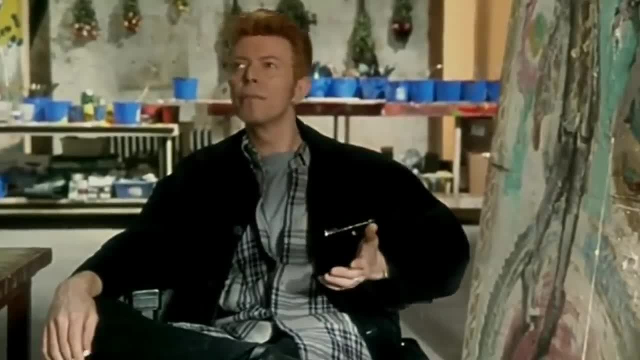 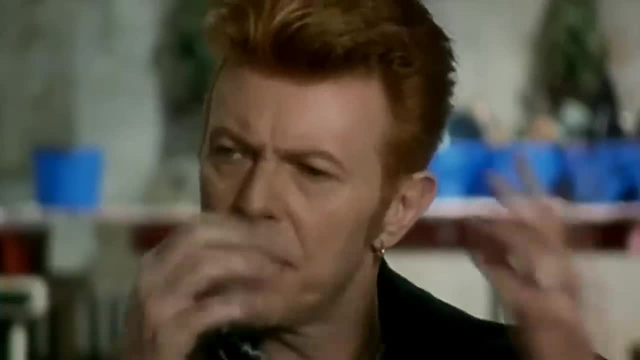 And it's something that I find very uplifting and optimistic and creative about working and being very much in the daylight. If I found myself in some kind of cul-de-sac in the music, I'd break down the problem by actually painting it. 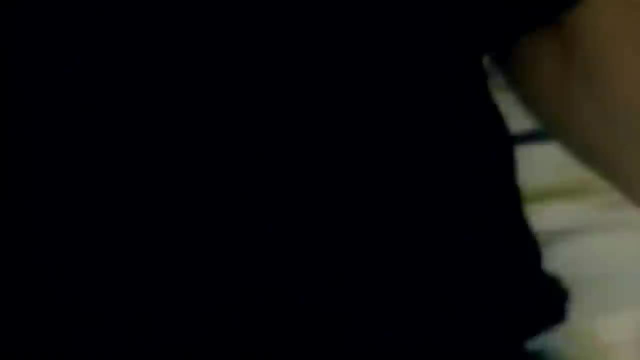 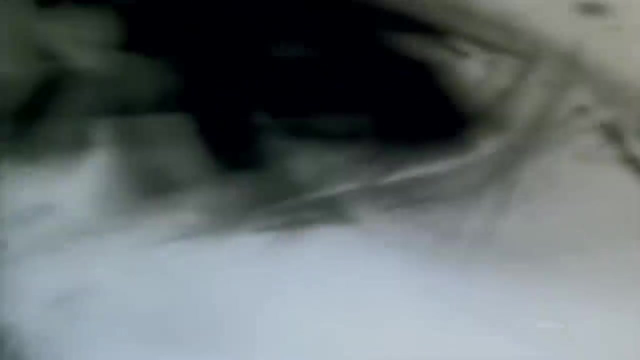 I'd try and visualise what the problem was, that the sense of these textures were grating against each other in a way that wasn't admirable, And I'd try and visualise those textures and paint them and then find out what was wrong. 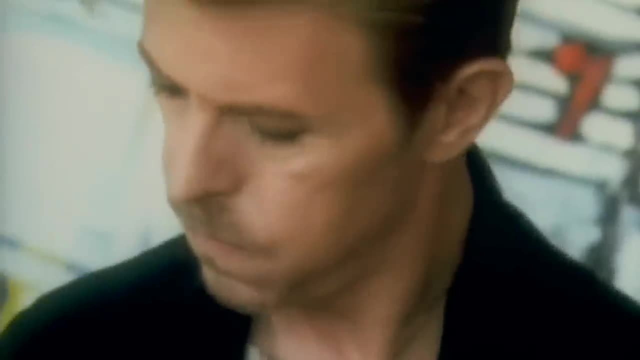 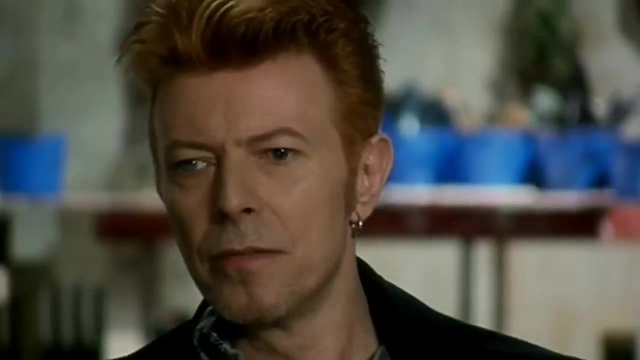 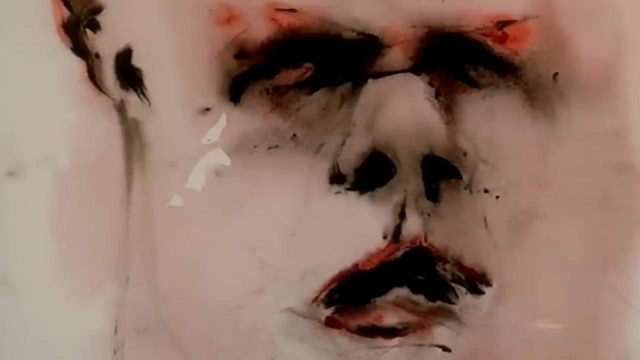 And then, when I'd solved that problem, I'd take it back into the studio. I've never really compartmentalised things. Everything for me is just this flux of doing stuff. Some of it's music and some of it's visual, And the two have always been very entwined. 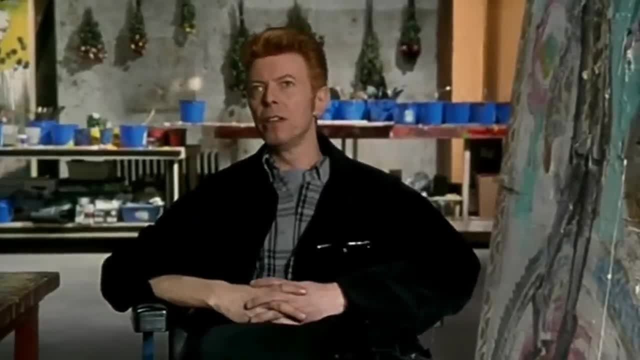 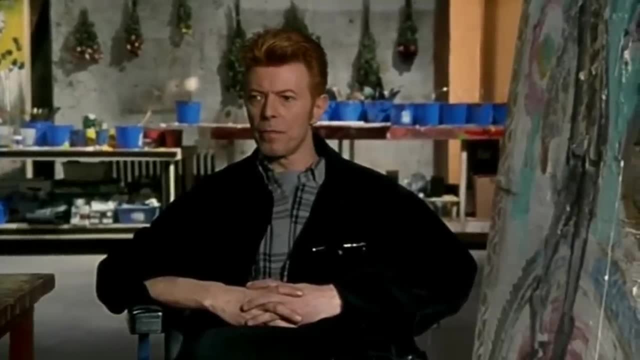 It's going to affect me, whether I like it or not. I'm going to be pained by the people that don't like it, and I'm going to be bolstered by people who do like it. What it won't do is change the way that I work. 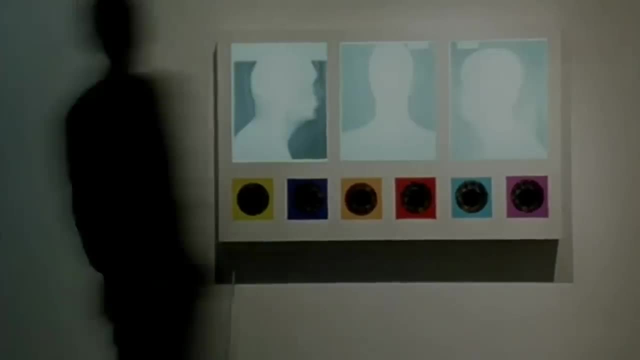 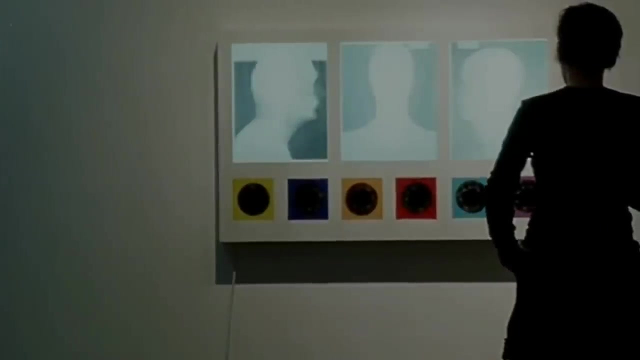 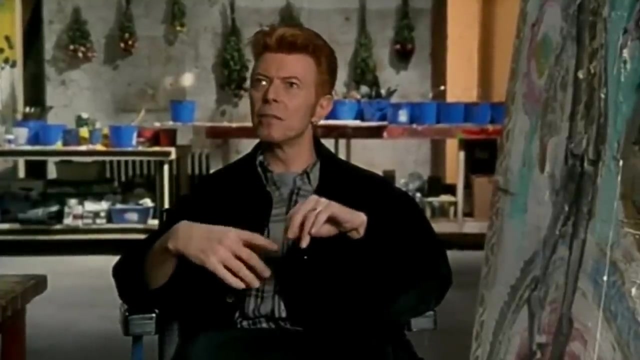 which is probably the most important thing. But whatever I hear- and people will insist on sending me any criticism- I'll get over it fairly quickly. I'm not thick-skinned, but I'm not thin-skinned either, But I've gotten used to the fact that you just can't please all the people all the time. 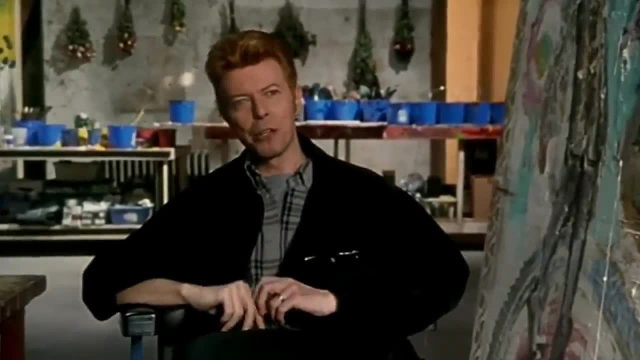 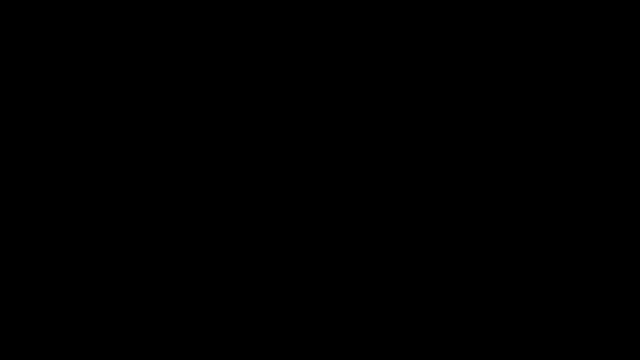 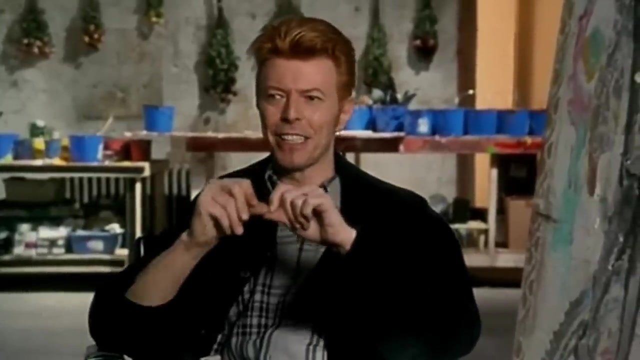 I've got no great desire to be loved in a major way by faceless, anonymous crowds. It doesn't really. It's not part of something that I want. Yes, never play to the gallery, I think, But you never learn that until much later on, I think. 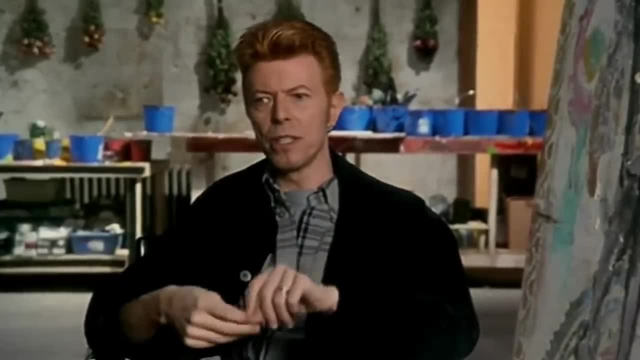 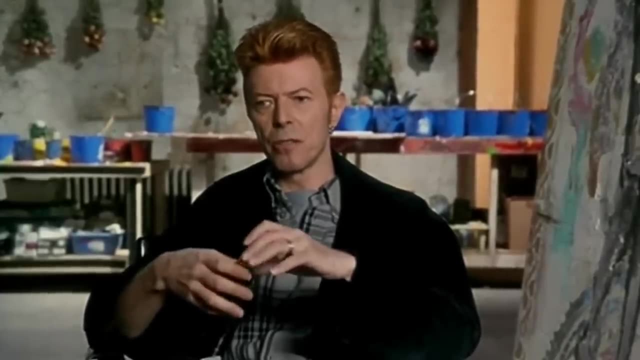 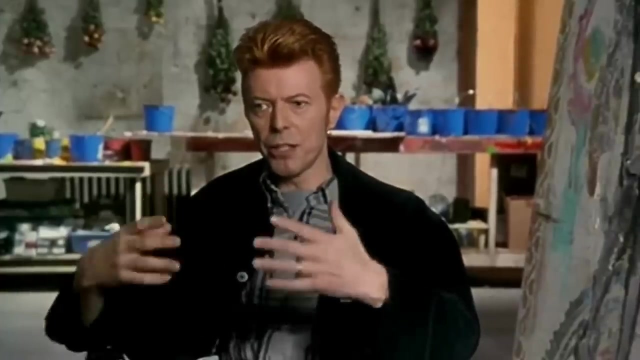 But never work for other people in what you do, Always, Always, remember that the reason that you initially started working was that there was something inside yourself that felt that if you could manifest it in some way, you would understand more about yourself and how you coexist with the rest of society. 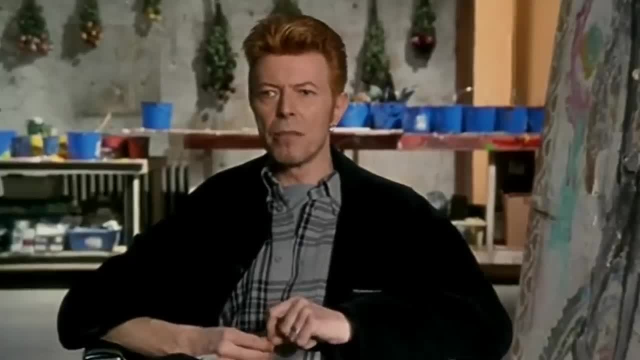 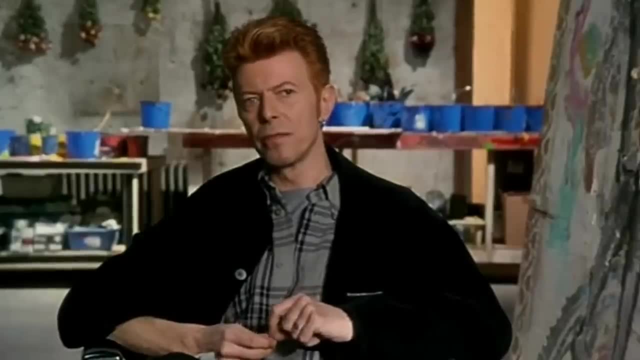 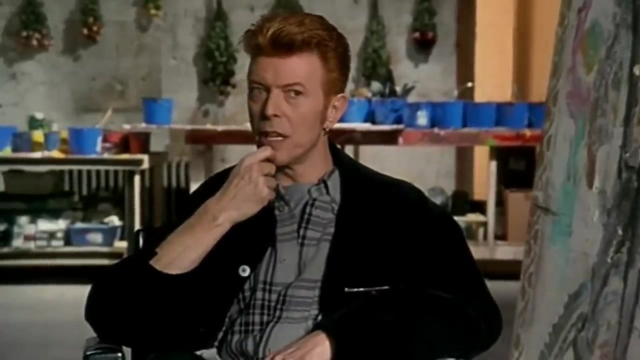 And I I think it's terribly dangerous for an artist to fulfil other people's expectations. I think they generally produce their worst work when they do that, And the other thing I would say is that if you feel safe in the area that you're working in, you're not working in the right area. 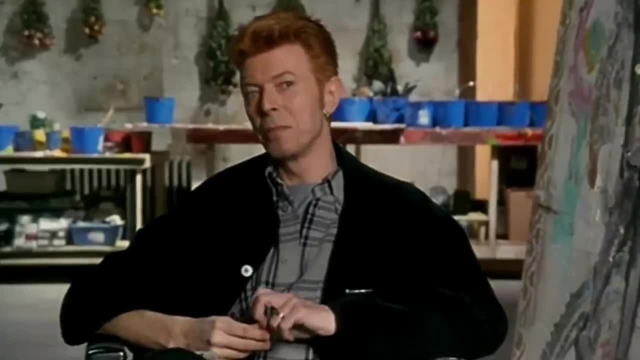 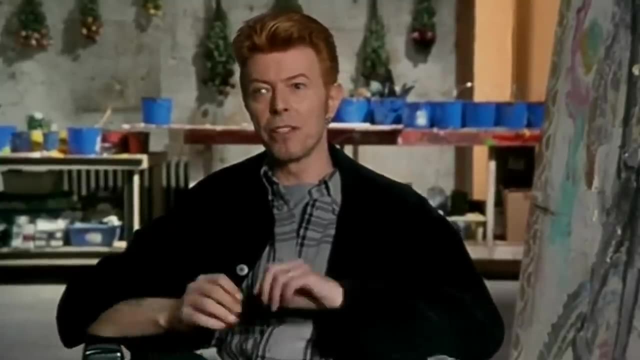 Always go a little further into the water. Then you feel you're capable of being in. Go a little bit out of your depth, And when you don't feel that your feet are quite touching the bottom, you're just about in the right place to do something exciting. 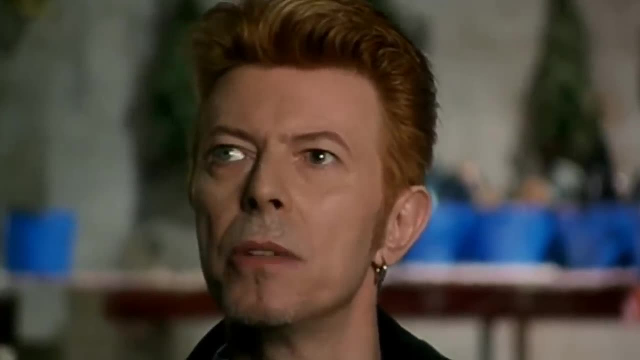 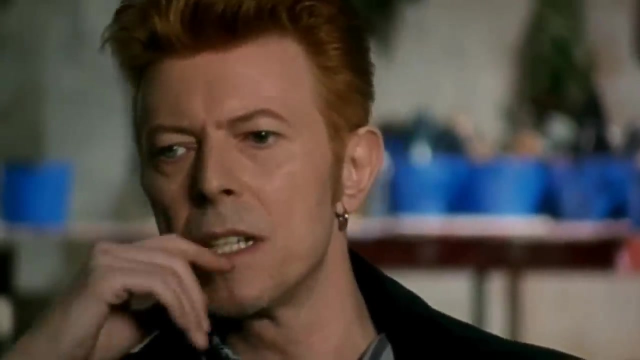 I wish I could be altruistic and say, no, it's just for the moment. But I kind of, I kind of I would like to feel, especially in music. I would love to feel that what I did actually changed the fabric of music.